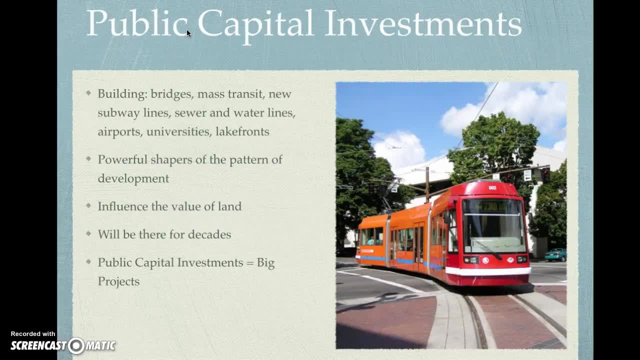 things you're gonna build. This is your bridges, your mass transit systems, new subway lines, entire sewer and water systems. We're talking things like airports, universities, lake fronts, as in you know, like Riverside developments. We're talking about these like really big projects or what we're. 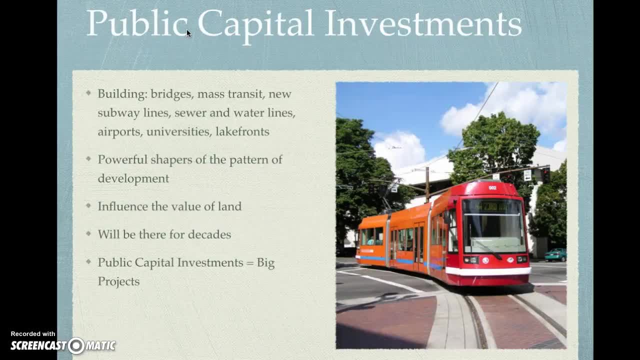 talking about is public capital investments. These are powerful shapers of the pattern of development. These type of projects influence the value of land. They're definitely connected to land value. What you build kind of dictates how valuable the land is gonna be, or what you don't build We're talking about. 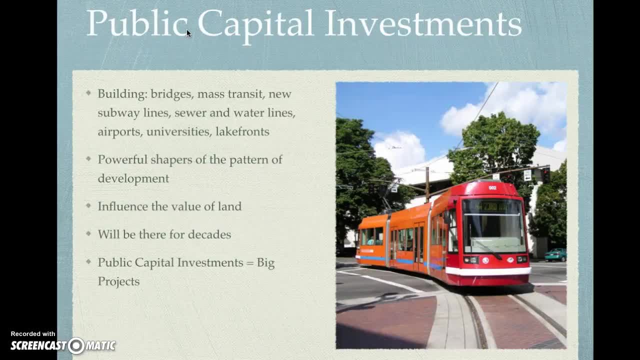 things that are gonna be there for decades, you know. so these are really visual decisions that we're making. These aren't just, you know, the stuff you're gonna see. It's stuff that's gonna be in a community for a long time. So really you could think of public capital investments means big. 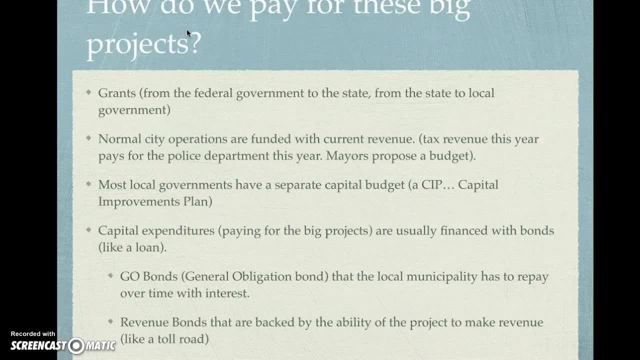 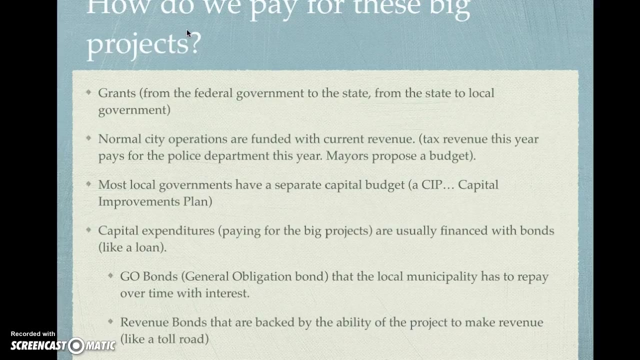 projects. So how do we pay for these big projects? One is grants. The federal government gives money to the state government. The state government then trickles it down to local governments. so one way is to get some federal funding, some grants. Normal city operations are funded with current revenue, like the tax. 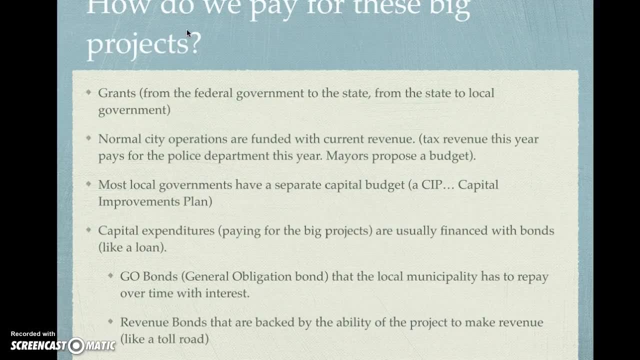 revenue this year pays for the police department. this year The mayor's proposed a budget. This is kind of like your normal city operations funded with revenue. now that's different than these public capital investments. there's a separate budget. governments have a separate capital budget, a CIP, a. 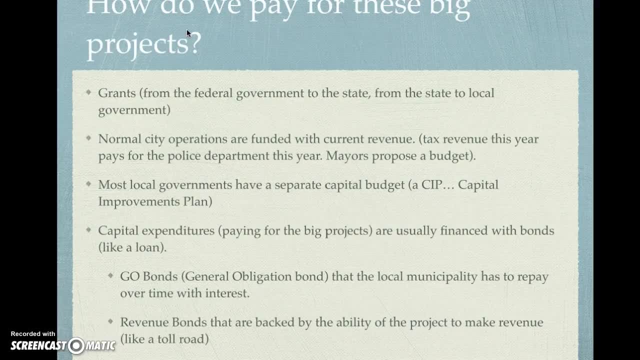 capital improvement plan. so this isn't like your normal operating revenue. it's the separate capital budget. so the capital expenditures, the money to pay for the big projects, is usually financed with bonds. that's kind of like a loan. two different kind of bonds are go bonds, the general obligation bond, and 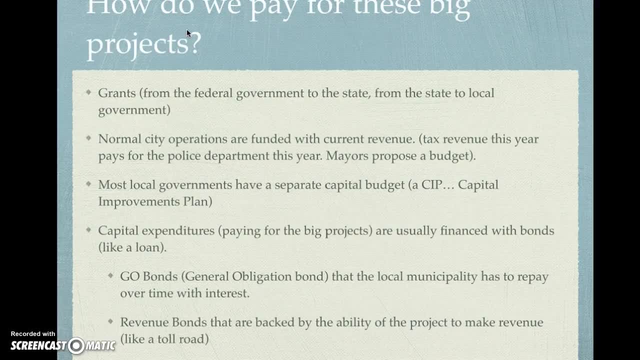 that the local government, the local municipality has to repay them over time with interest. or there's a revenue bond which is backed by the ability of the project to make money, to make revenue. so that type of bond is like- think of it like a toll road, you know, like if you build the toll road it's like you're. 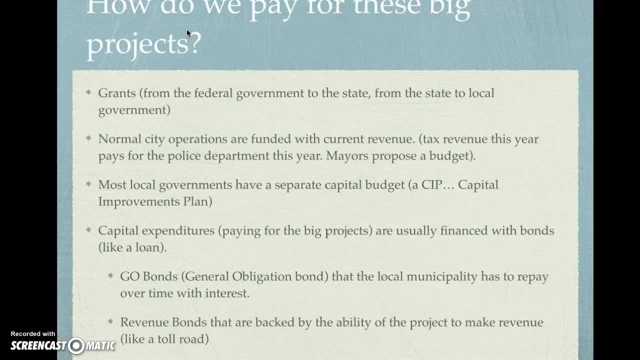 building the road and you know you're gonna collect tolls to pay for the road. a bond is a toll road and you know you're gonna collect tolls to pay for the road. to you know, for something like that, that you know it's a project that you can. 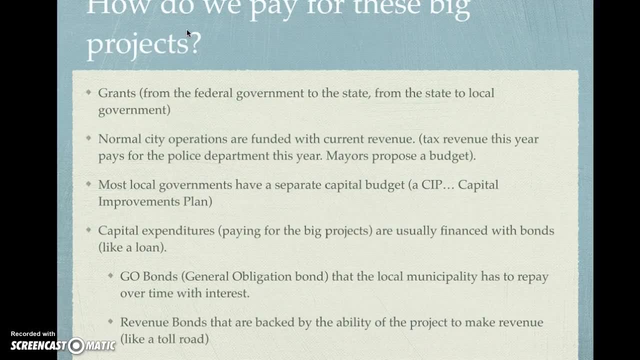 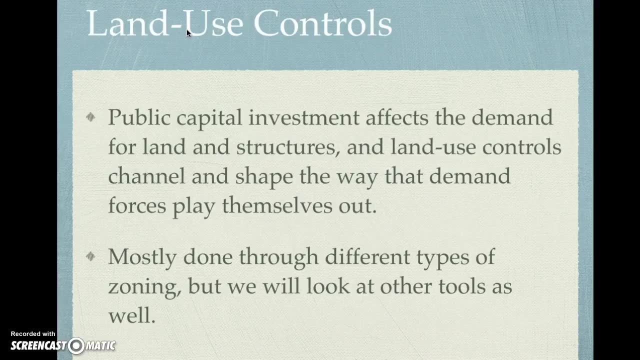 kind of link that it's gonna make money. so those are the kind of type of bonds I mean. that's how, that's how we pay for these big projects. a lot of money involved here. so land use controls. we're kind of switching gears now. so if public capital investments, if those big projects affect, 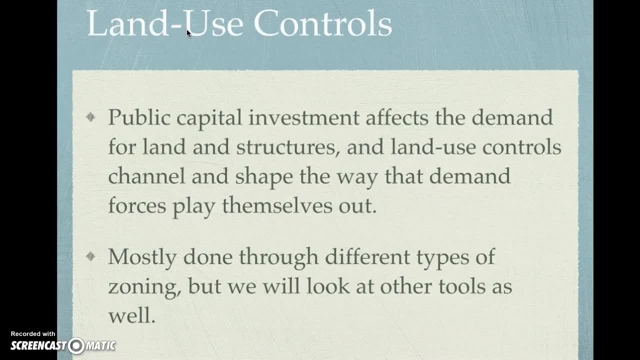 the demand for land and structures. land use controls are what's going to channel and shape the way that those demand forces play them selves out, and this is mostly done through different types of zoning. we're gonna look at a couple other tools, but just we're not gonna go too far into. 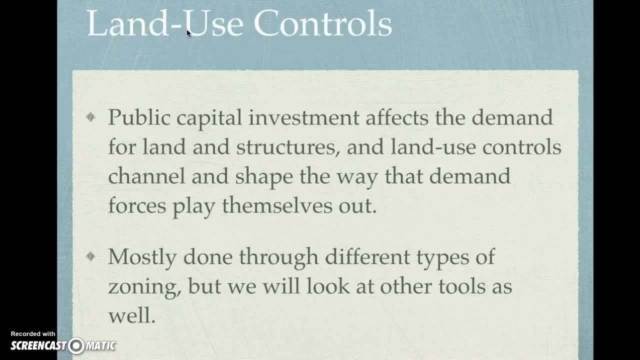 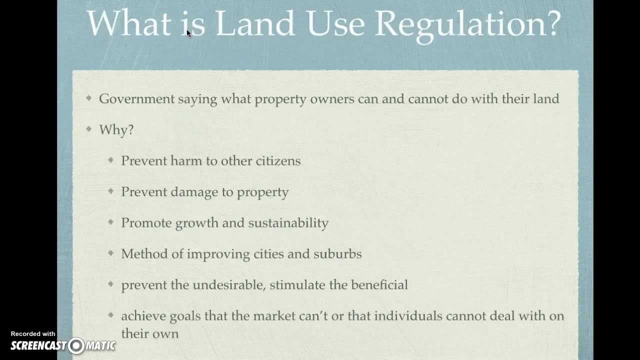 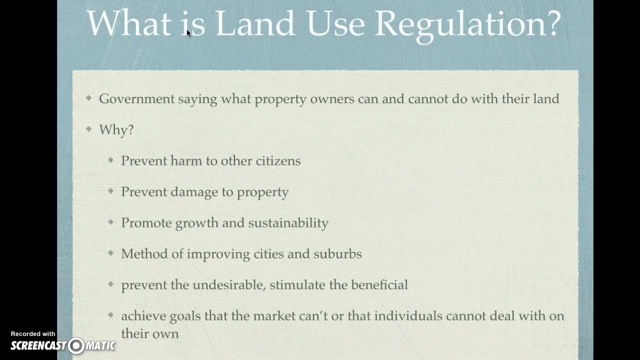 zoning, because here at Dillard we have an entire land use policy class, but we're just gonna kind of briefly get it into our heads about what zoning is, what it can do. okay, so before we dive into zoning like as a tool, what is we're talking? land use regulation? we're talking about how. 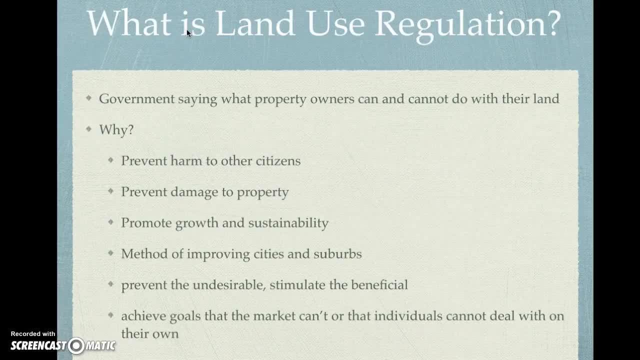 we shape land, what we can do, so really, this has to do with the government saying what property owners can and cannot do with their land. that's kind of what we're talking about with land use regulation. so why, like why, would the government get involved with saying what private property, like owners, can do with? 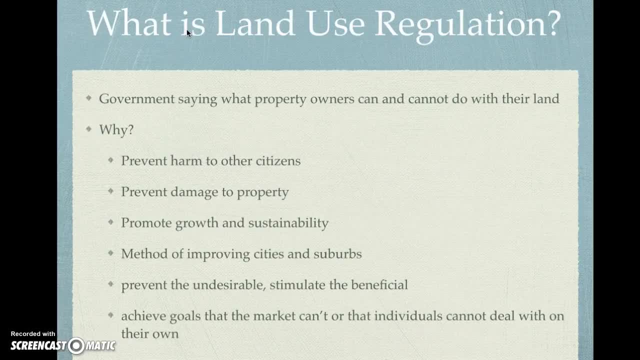 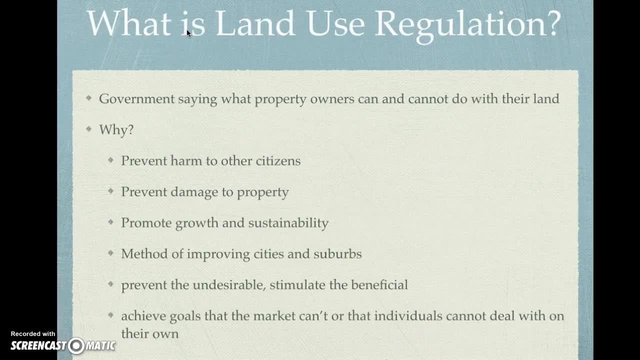 revitalization. it's really. it's kind of like you start controlling the use of land, saying what you can and cannot build on certain areas of land is to prevent the undesirable and stimulate the beneficial. it's kind of like an overall goal and also the government gets involved with regulating land. 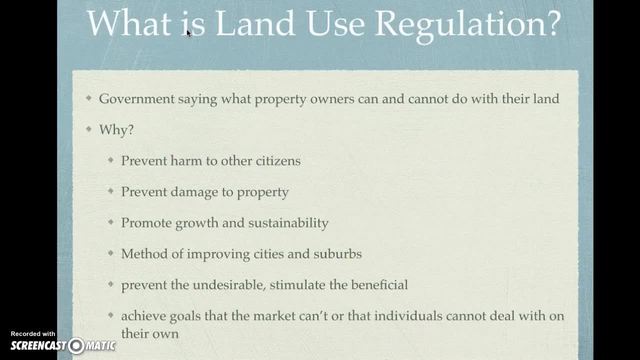 because you need to achieve goals that the market can't, or we're talking about something that individuals can't deal with on their own. I mean, just think about the, the magnitude of these capital investment projects we talked about. I mean, these are like, these are too big. 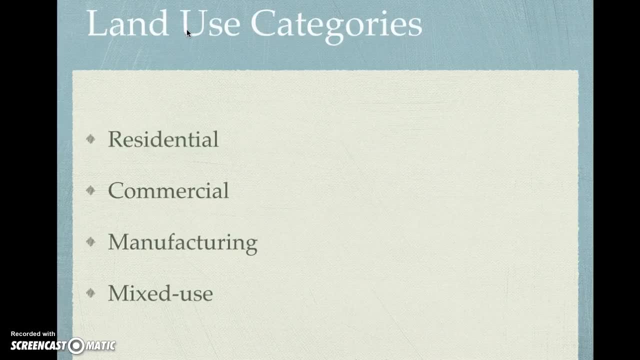 like individuals can't deal with these things on their own. so just to give you an idea, when we say land use, I want you to know some different categories. I mean, basically, when you're talking about chopping a city up into pieces and saying what you can use the land for, these are gonna be your categories. it 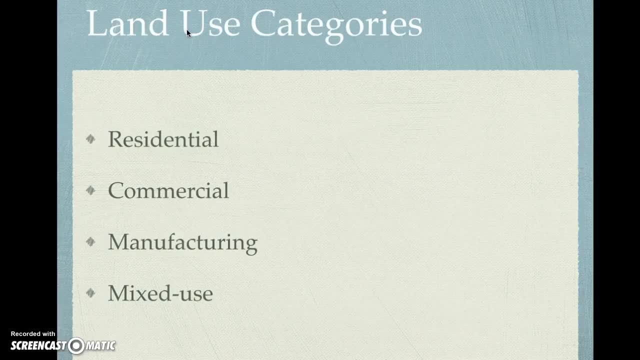 can be residential houses. it could be commercial. this is your businesses, your commercial activity: manufacturing, yes, and mixed-use. mixed-use is well, it's kind of like it sounds it's a mixed of uses. this is like I always envision the building that's got like the store on. 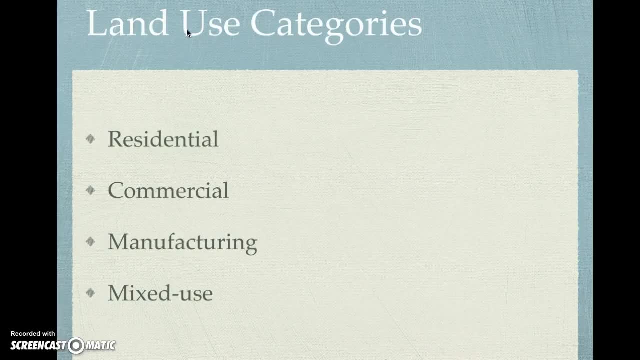 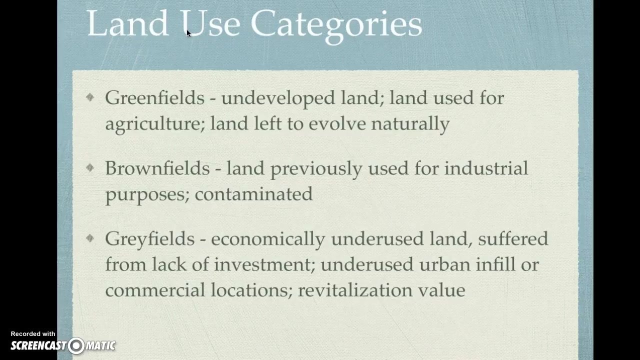 the bottom and the apartments on the top. so these are your basic categories of how to use land: residential, commercial, manufacturing or a mixed-use type development. so a couple other words that I want you to know different land use categories, that these are that are used in urban planning, and I want you to know them so you can feel. 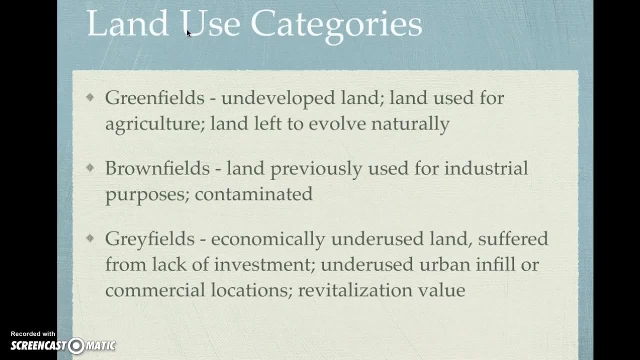 fancy one is called green fields- sorry, I always have to pause to take a drink- and green fields are. this is your green space, your undeveloped land. it's land that's used for agriculture. it's land that's left to evolve naturally- your green, green fields. the other one is brown fields. this is land that was. 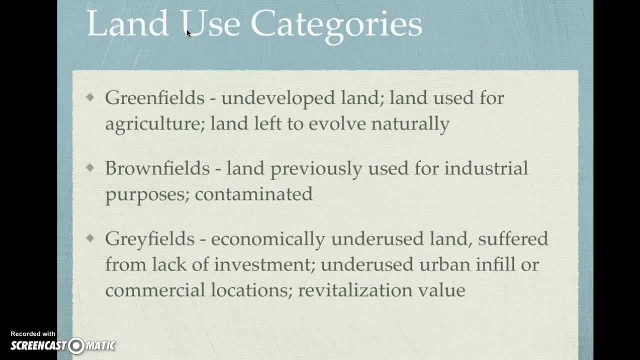 previously used for industrial purposes. this is like your contaminated land. this is your dirty, nasty, polluting factory that's not there anymore, so the spaces that are left behind are called brown fields, and then you have something called gray fields, and this is economically underused land. maybe it suffered from a lack of investment. it's 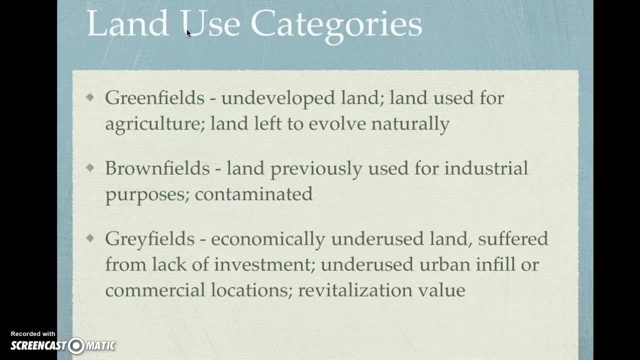 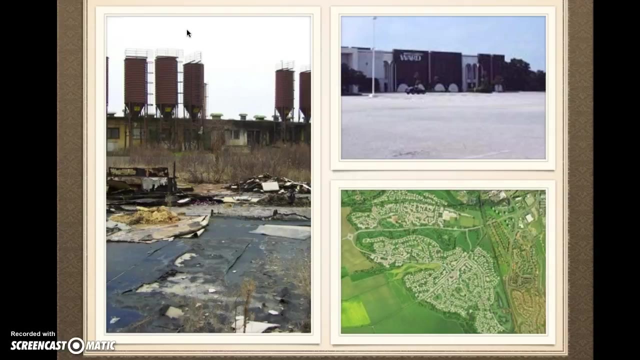 an underused, like urban infill or commercial locations, but it's something that maybe has redevelopment or revitalization value. so, green fields, brown fields, gray fields- here's a picture of what some of those would look like. so, on the left, you've got your your brownfield. this is this industrial. 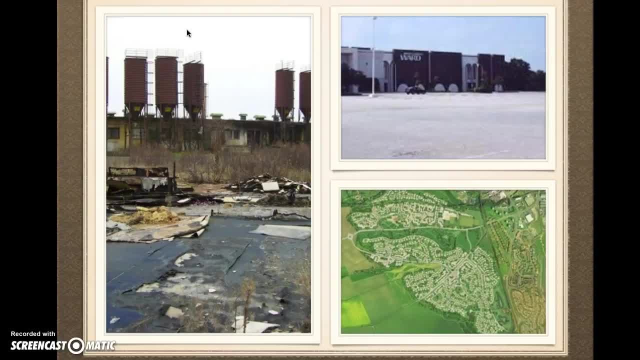 site. it used to be kind of an industrial manufacturing site. now it's kind of like this big contaminated area in the top right hand corner that would be like a gray field. see how it's like a shopping plaza. maybe it's underutilized, kind of suffering from disinvestment. I mean you got a huge parking lot with no cars in. 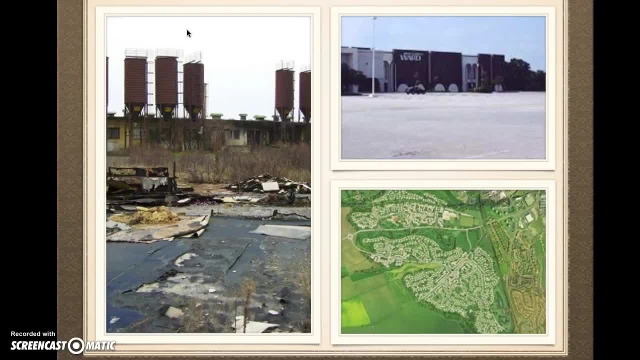 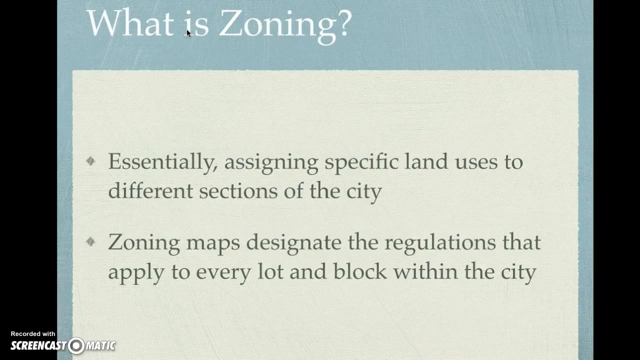 it. that would be like a gray field and then on the bottom is more of like a green field where you've got the green spaces, kind of like the underdeveloped layer, the undeveloped land. so this is just some of your examples. okay, so zoning, and quickly. what is zoning? essentially, what zoning means is you're. 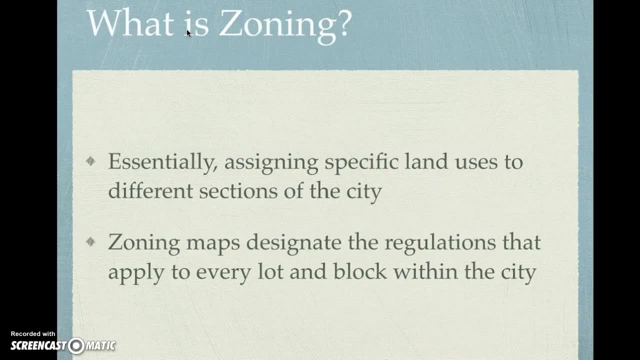 assigning specific land uses to different sections of the city. you've got a map. it chops the city up into different zones and they designate the regulations that apply to every lot and block within the city. so you get a map of the city segmented into zones. say what you can and cannot do. 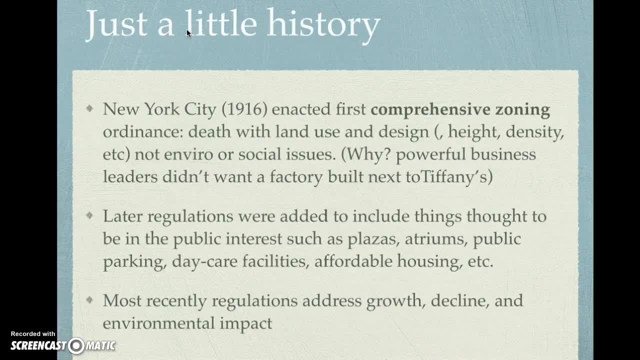 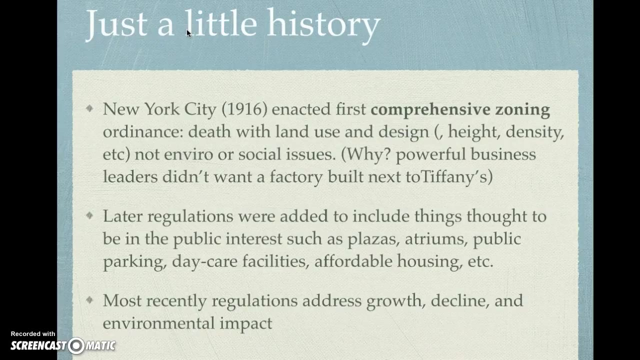 specifically in each zone. just a little bit of history about zoning. so New York City enacted the first comprehensive zoning ordinance that says death. it should be dealt. I'm sorry it dealt with land use and design. this is things like height, density of buildings. we can talk about that in class, but it didn't really. 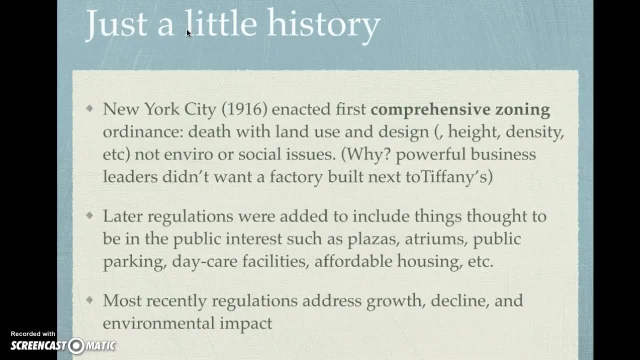 focus on environmental issues or social issues. um, it came about why? because really think of this. like these, powerful business leaders in New York City didn't want a factory built next to their fancy stores like Tiffany's. so that's kind of how zoning came about. later, different regulations were added to include 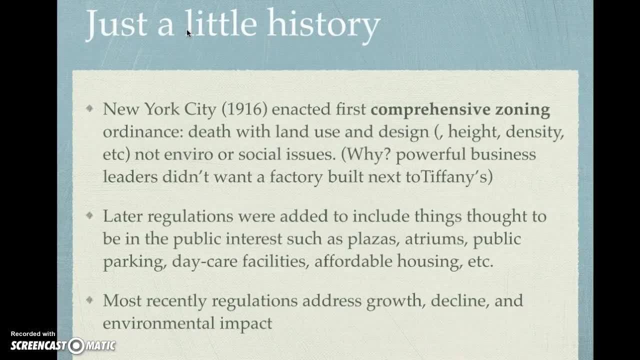 things that were thought to be in the public interest, like plazas, atriums, this parking, daycare on public spaces. so, and then, more recently, we've started addressing population growth, city growth, cities in decline, and then environmental impact. so zoning ordinances, this is your best known form. 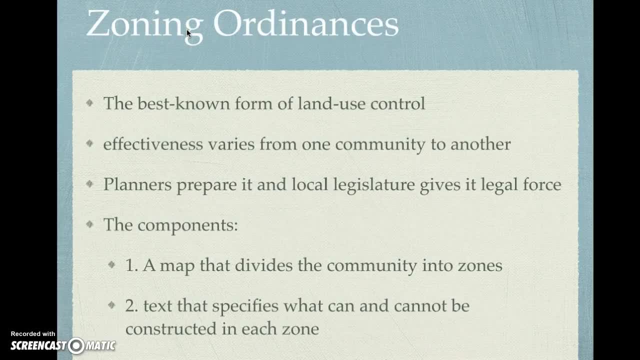 of land use control, the effectiveness of zoning ordinances, that that's gonna vary from one community to it, to the next. planners prepare it and then local legislators give it legal force. so with a zoning ordinance in New Orleans it's the CZO- comprehensive zoning ordinance. the components are based. there's basically two components. one- you've got a map that-